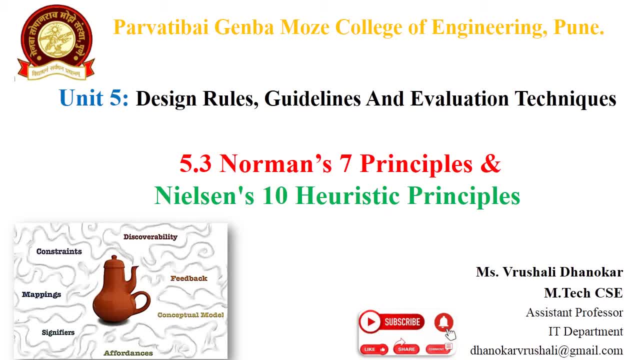 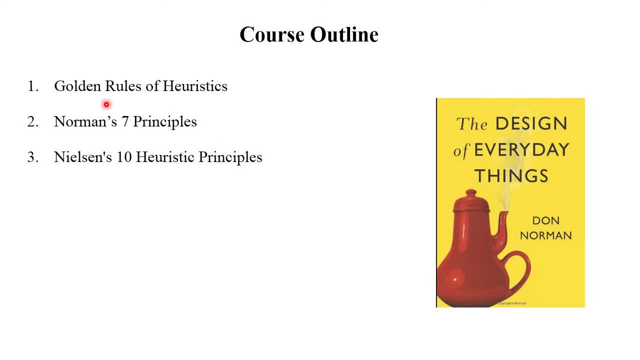 So let's see how exactly these principles will be work Next. Following points are covered in this video, which includes Golden Rules of Heroistics, Normal 7 Principles and Nelson's 10 Heroistic Principles. So let's see The first Golden Rules of Heroistics. 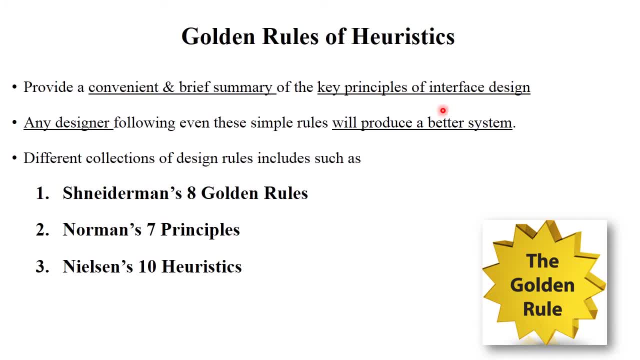 It provide a convenient and brief summary of the key principles of interface design. Any designer following Even the simple rules will produce a better system. There are different collections of design rules, which includes such as Snyder Man's 8 Golden Rules, Normal 7 Principles and Nelson's 10 Heroistics. 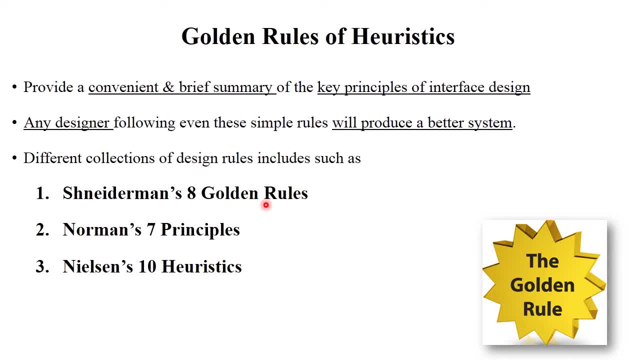 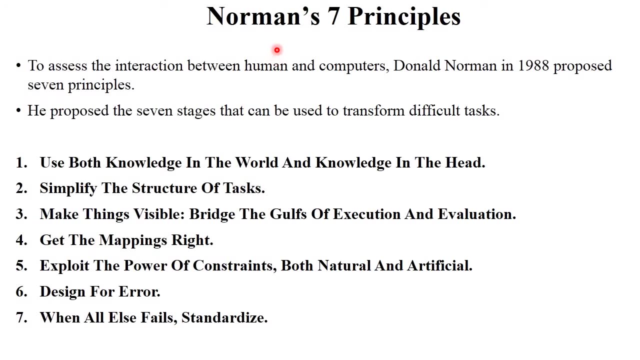 I have explained with examples Snyder Man's 8 Golden Rules in my last video. Now in this video we will learn Normal 7 Principles and Nelson's 10 Heroistics. So let's see The first principle, That is, Normal 7 Principles. 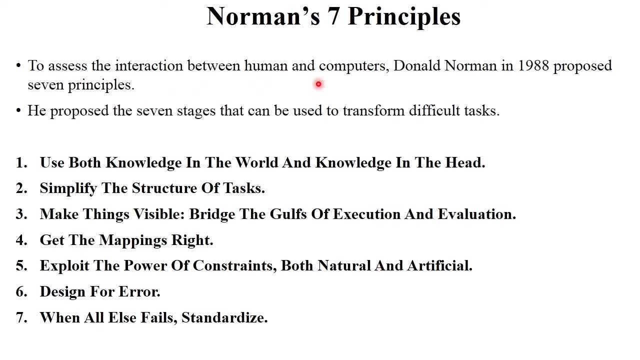 To assess the interaction between human and the computer. Donald Norman in 1988 proposed 7 principles. He proposed the 7 stages that can be used to transform the difficult task into the simple task Right. Each and every designer. Designer will use all those principles for implementation or for design a particular product or particular system. 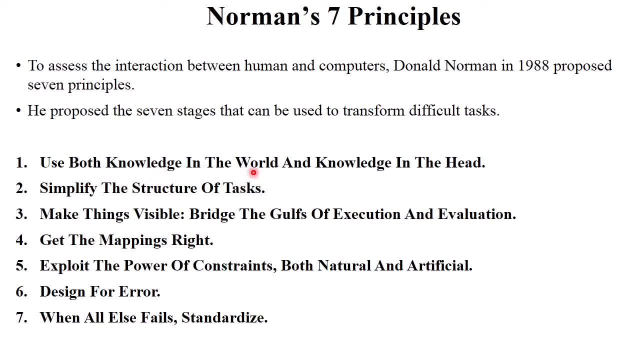 The first principle is: use both knowledge in the world and knowledge in the head. Next, simplify the structure of task, make things visible, get the mapping right, exploit the power of constraints, both natural and artificial- design for errors and, when all else fails, standardize. 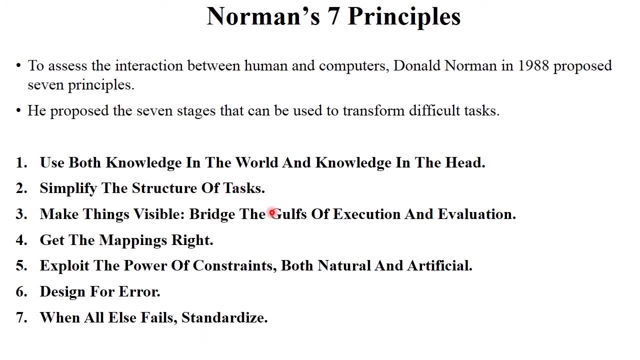 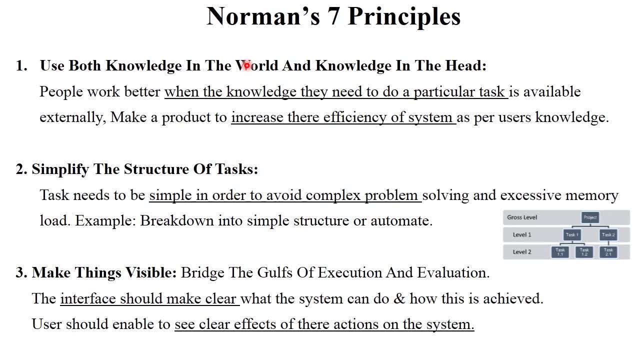 So these are the Normal 7 Principles. Let's see how exactly these principles will be work Next. So the first Normal 7 Principle is: use both knowledge in the world and knowledge in the head. It means that people work better when the knowledge they need to do a particular task is available externally. 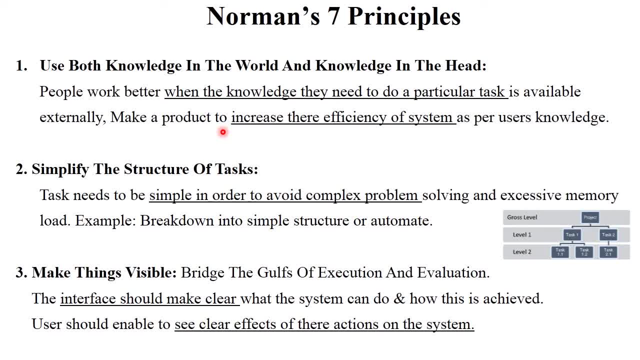 Suppose, for example, we all are familiar with different social apps, right, We easily use those things. Suppose user familiar with the features of the particular application, So it makes easy To perform a particular task, Right? So at that time it increase the efficiency of systems. or as per the user's knowledge, 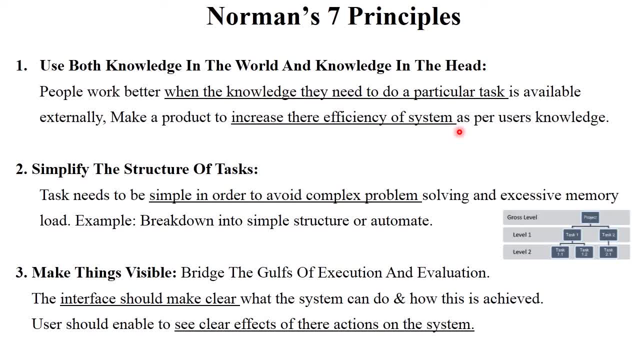 Clear- Suppose, for example, WhatsApp- We all are familiar with that- how exactly chatting application will be work, the audio call, video call, then a posting, a different types of status, Right. So we all know how exactly this system works. 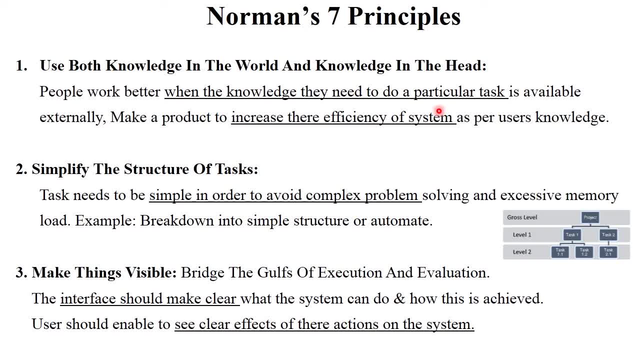 So users get easy access to the system And it will be easily available. on that It increase the efficiency of system as per the user knowledge right. The next principle is simplify the structure of task. Task needs to be simple in order to avoid a complex problem. 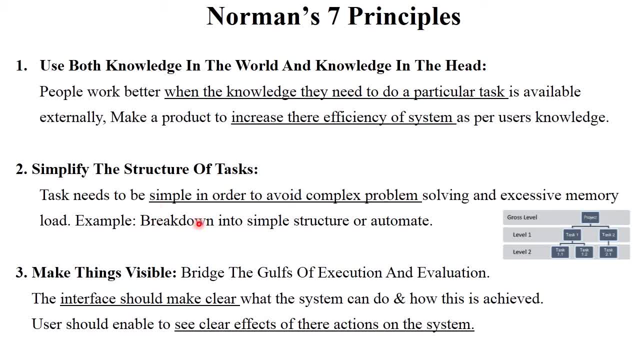 It's sort an excessive memory load, For example, a breakdown into simple structure or automate. We all are familiar with Microsoft Word. In Microsoft Word, there are different types of menus available. That is, few types of menus can be available, For example, Google, Google, zwMP. 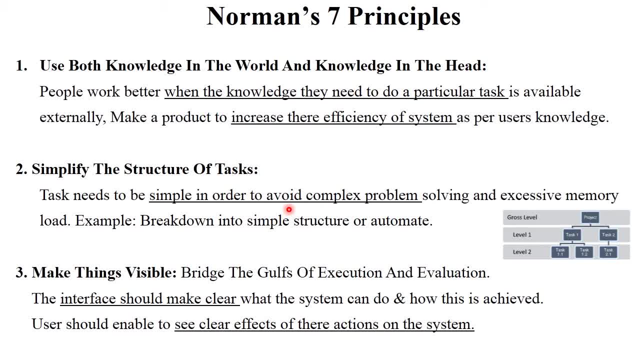 that is, file, edit etc. so in file there will be a new. then say: say: as this kind of option will be available, right next edit, edit, include, cut copy paste, undo this kind of option available. so it's easy to use as per their clusters or as per their features. so task need to be simple in order that. 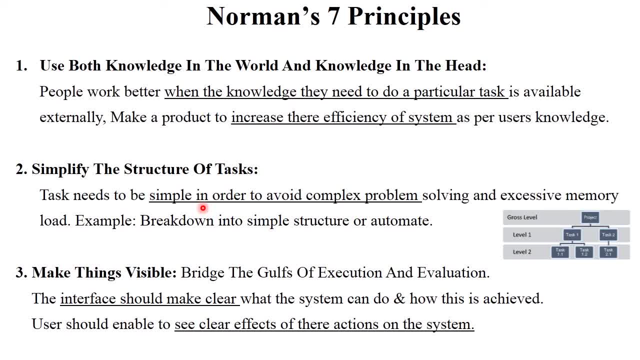 is technical, non-technical persons use those application clear. the next principle is make things visible. it means that the interface should make clear what the system can do and how this is achieved. user should enable to see clear effects of their actions on the system. right, you should. 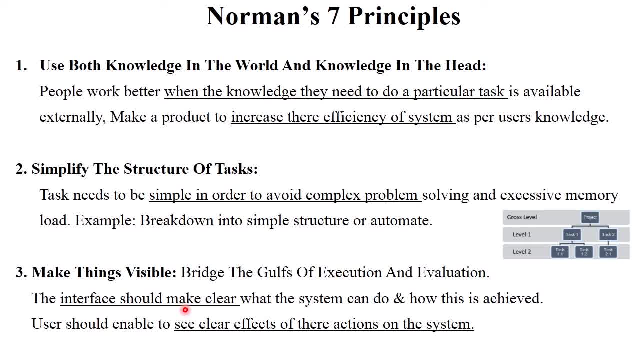 visit a particular website or the shopping website. so their interface should make clear whether the james, james and lady were right. so their interface should make clear there are particular payment method, payment option, different types of discounts are available so we can easily watch or easily use or access the particular website. right user should enable to see clear effects of their action. 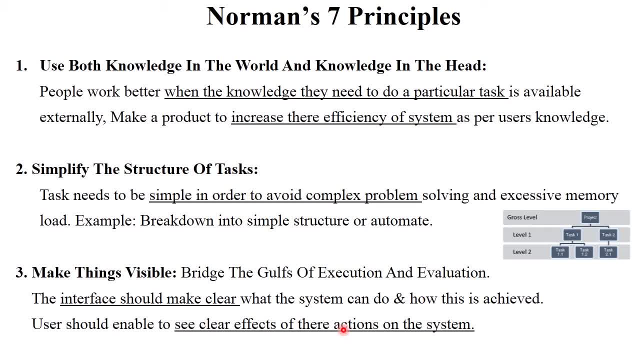 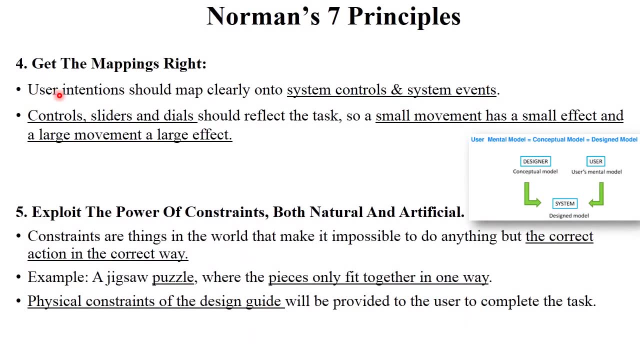 suppose user press the submit button, the particular task will be submitted right. so user know that how exactly happen on that particular screen, right? so this will make things visible. next. the next principle is get the mapping right. it means that user intention should map clearly on to the system controls and system events. 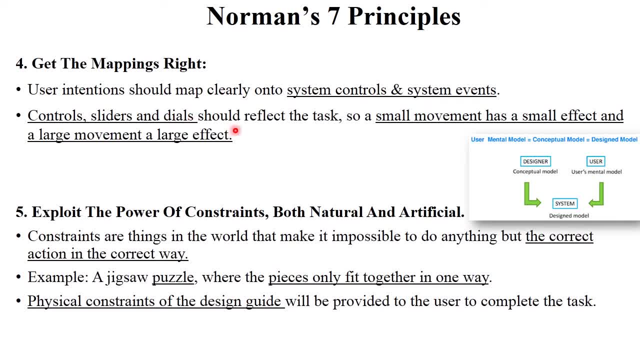 decrypting just list of bytes should reflect the paths. the small moment has a small ethics and large movement a large effect. this user handle a particular system so you can know back a user understand to this instance is very important. intention can also affect the user features. pedestal details and buttons처�. 엄 exhausts under randomに. 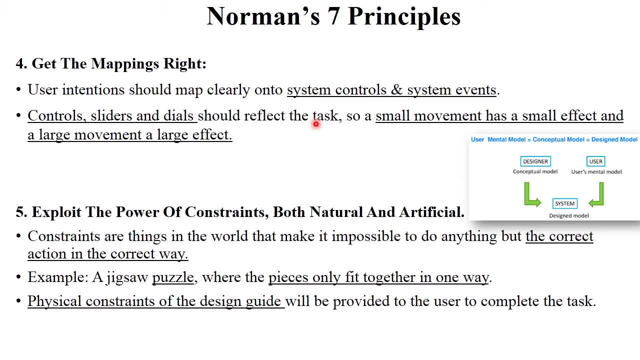 certain system controls are displayed on the nachoANSI manual or cigเห� 00 verz sealed model. so user know that over, user understand the" that how exactly particular system will be work. So, as per their understanding, as per their knowledge, user handle a system controls as well as system events, Clear. 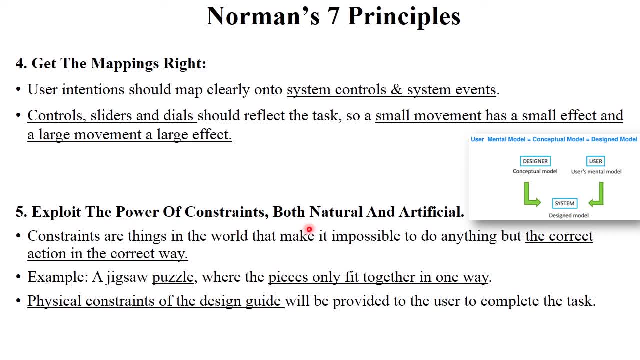 The next principle is exploit the power of constraints, both natural and artificial. Constraints are the things in the world that make it possible to do anything but the correct action in the correct way, For example, puzzles where the pieces only fit together in a one way: Right. 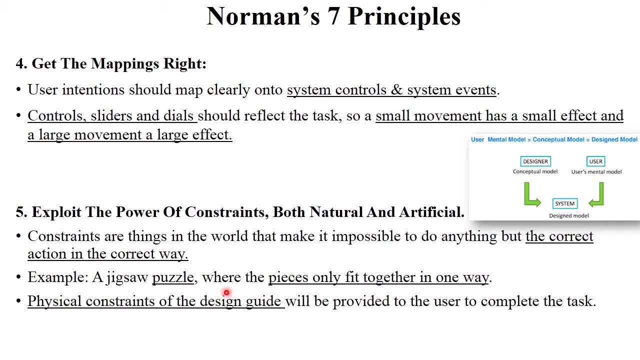 So user must know that how exactly it will be work. They have the knowledge or theorems regarding that Physical constraints of the design guide will be provided to the user to complete the task. For example, suppose a someone buy a washing machine, Right? So 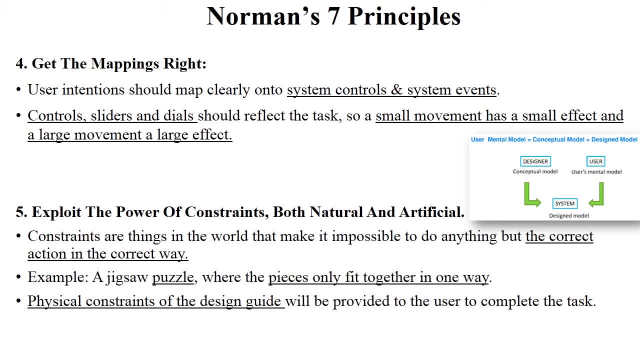 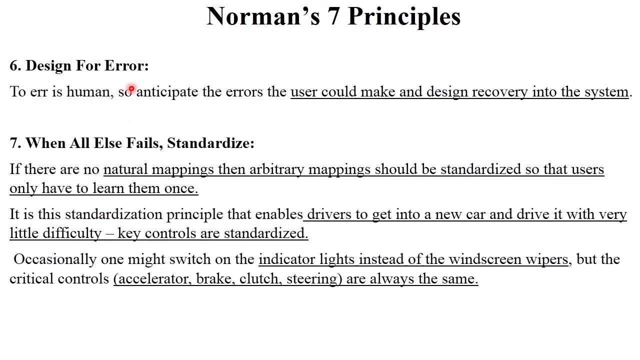 there will be a particular helping guide how exactly the particular function will be work Right. So particular design guide or helping guide will be provided to the user to complete a particular task. Clear Next. The next principle is design for error. To err is human, So anticipates the error user. 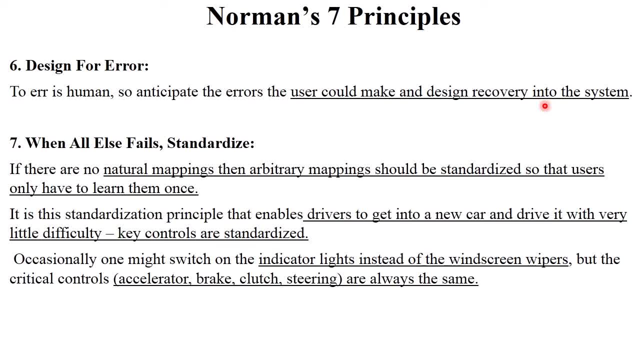 should make and design recovery into the system. Suppose you enter a wrong mail id, it shows the message. please enter your valid email id. Suppose you enter a wrong password: that will be stored into the system So it generates a message. please enter a right password. Right, So design for error. 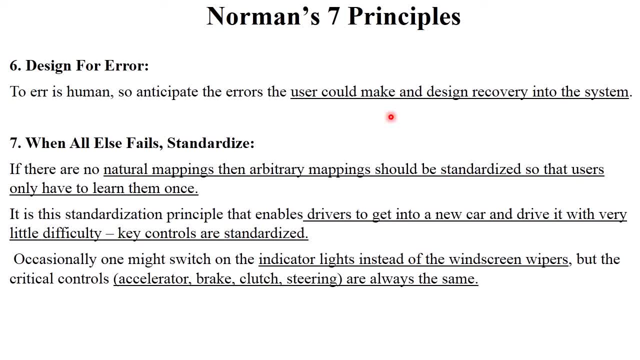 Means user could make and recover your system properly. And last principle is: when all else fail, standardize. If there are no natural mappings, then arbitrary mappings should be standardized So that user only have to learn them once. For example, there are different. 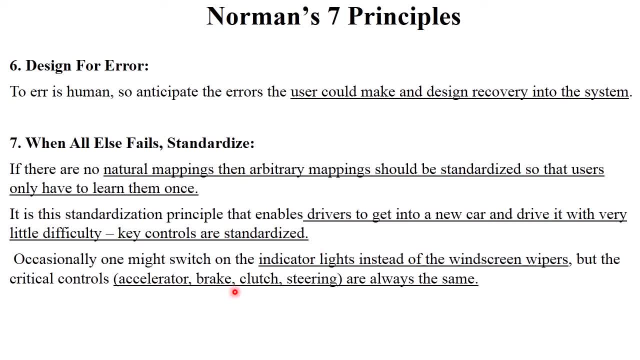 features of particular bike: Right: Accelerator, brake, clutch, steering. This kind of features are always same Right, But there are some new features are included in that particular vehicle. That is, indicators light instead of white screen wipers, So users get easily. 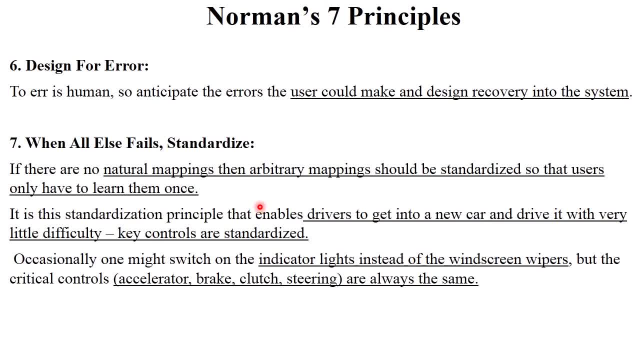 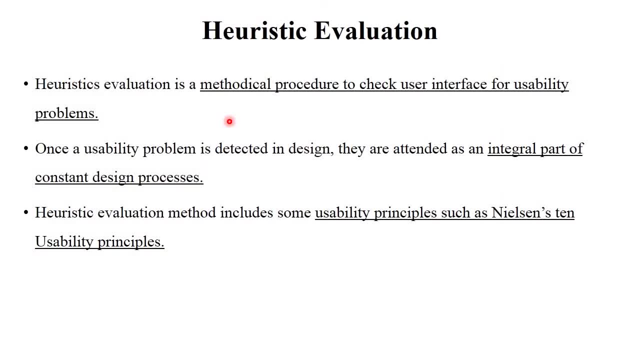 use those new features Clear. So this means that when all else fail, standardize Next. These are the normal 7 principles. Hope you understood to get easy to understand. The next, heuristic evaluation. Heuristic evaluation is a methodical procedure to check user interface. 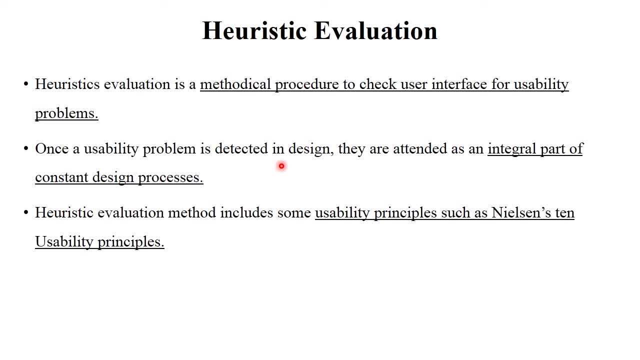 for usability problems. Once a usability problem is detected in design, they are attended as an integral part of constant design process. Heuristic evaluation method include some usability principles, such as Nelson's 10 usability principles. So this all principles- are generally used in design process. It's easy to implement or to get the requirements of these principles. 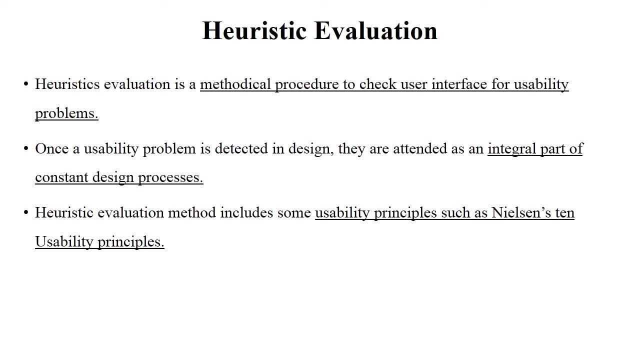 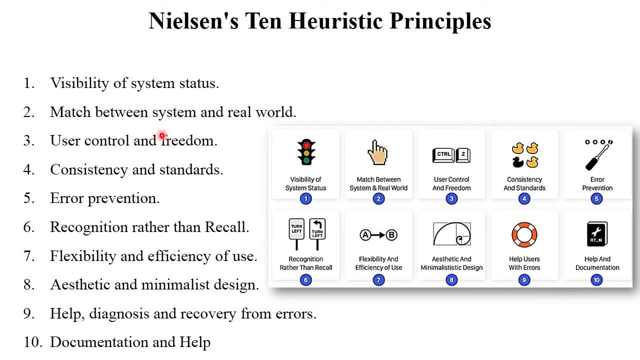 To get the requirements of the user or to make a particular system more useful, Right Next. So these are the Nelson's 10 heuristic principles. We all are familiar with that. First, visibility of system status. There will be a particular system status, That is, battery. 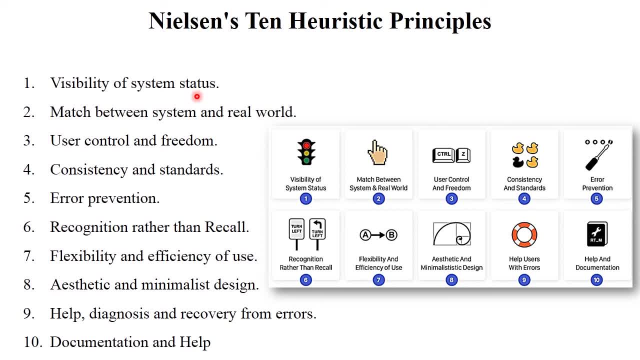 server mode, The particular application. switch on or switch off Right, So visibility of system status must be shown. Then match between system and the real world application, So the user control and freedom. It means to use different types of shortcut keys while using a particular application. Then the particular consistency and standard design. 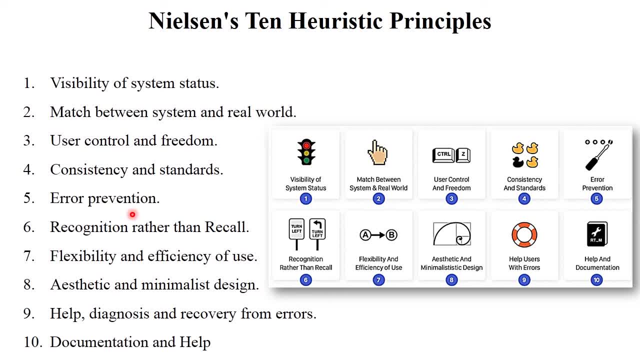 standard will be maintained: Error prevention, Recognization rather than recall. I have explained all those things in my last video, That is, Snyderman's 8 golden rules. Generally, these Nelson's 10 heuristic principles and Snyderman's 8 golden rules will be explained in this video. 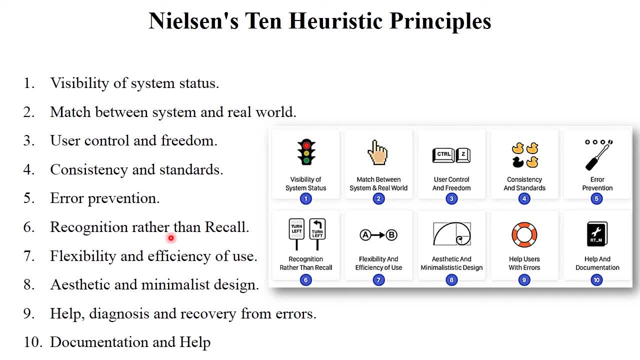 These golden rules will be most similar. Then, recognition rather than recall Means generally use short term memory to recognize a particular thing Right. Next, flexibility and efficiency of use. Assistive and minimalistic design Means generally is easy to use for each and every person. It helps diagnosis and recovery from errors and documentation. 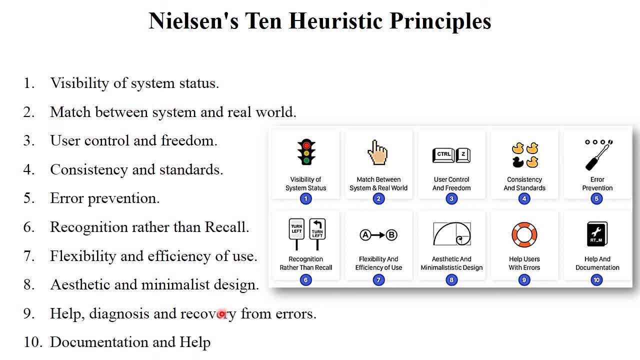 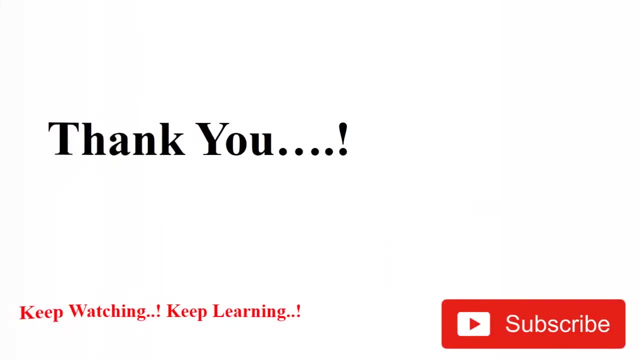 and health Right. So we all are familiar with all those things Because in general real world we use all those things while design, while using a particular application or the system Right. So these are the Nelson's 10 heuristic principles. Next, Hope so you.